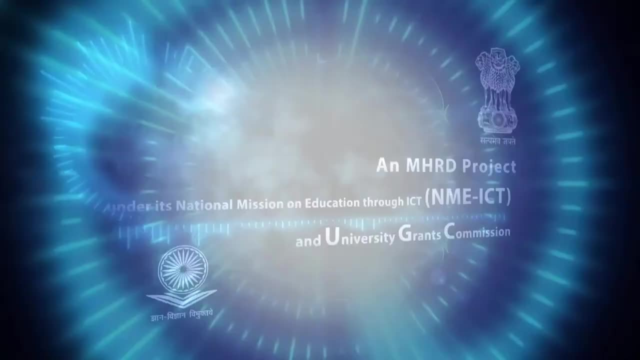 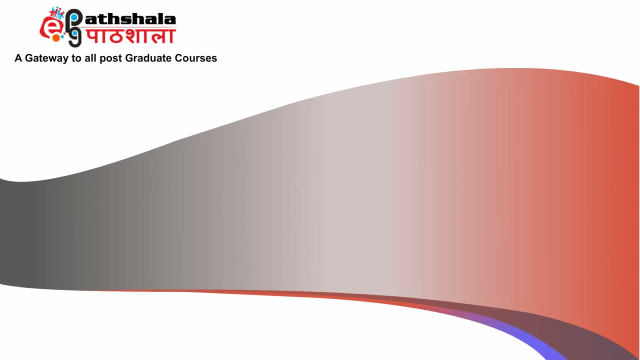 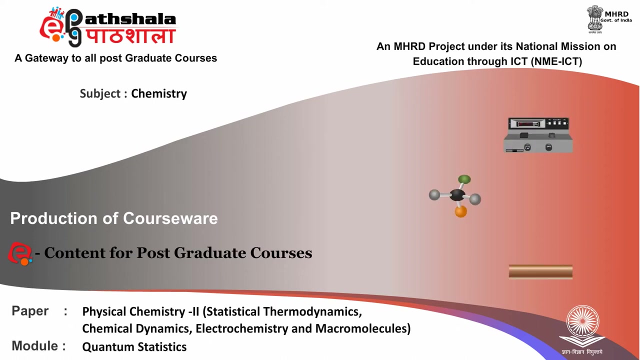 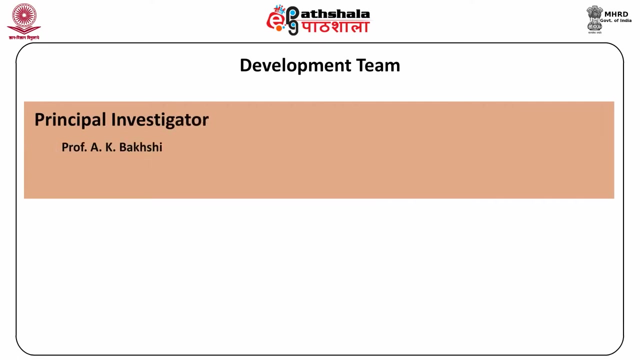 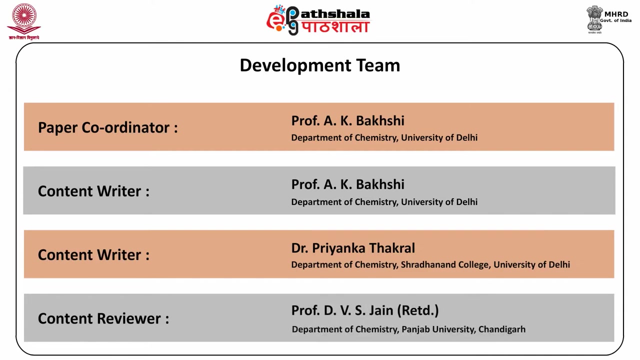 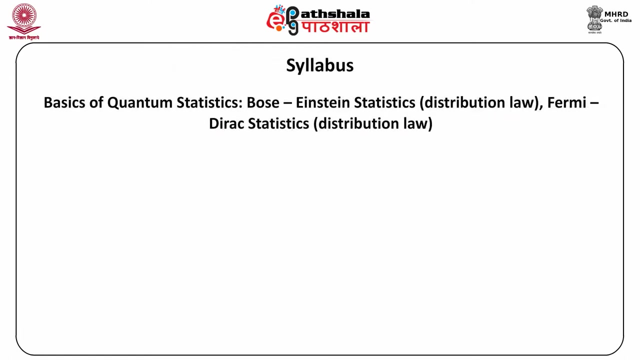 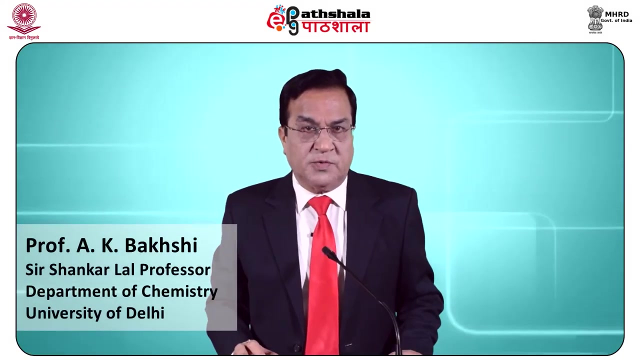 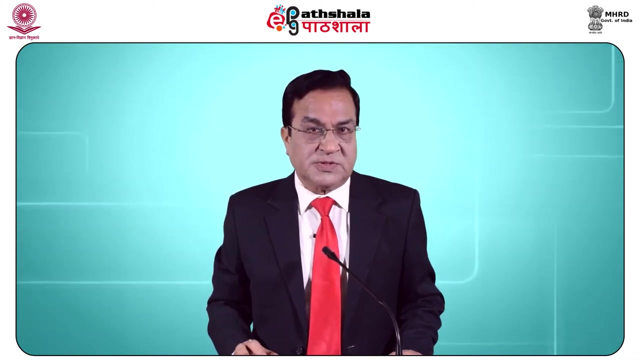 Thank you for watching. Thank you for watching. Thank you for watching. In the previous module we talked in details about the Maxwell Boltzmann statistics and we also derived the Maxwell Boltzmann distribution law. Maxwell Boltzmann statistics, as you know, is also called classical statistics. 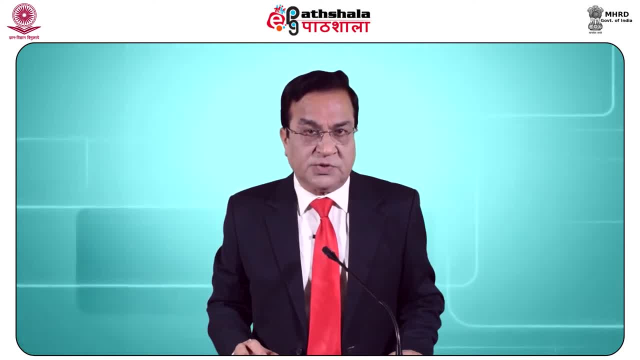 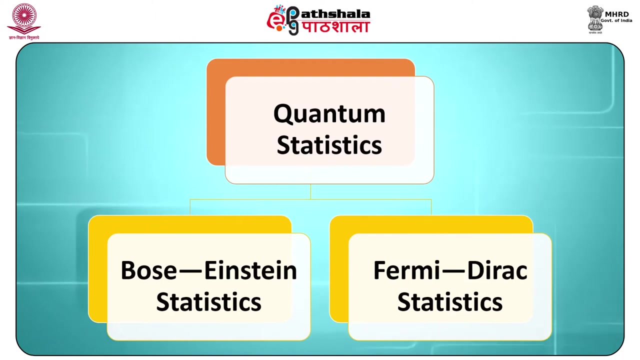 In this the particles are distinguishable from each other and there is no restriction on the occupancy of energy levels. Further, here we also do not take into account the internal structure of the particles. Today we will talk in detail about quantum statistics. There are two types of quantum. 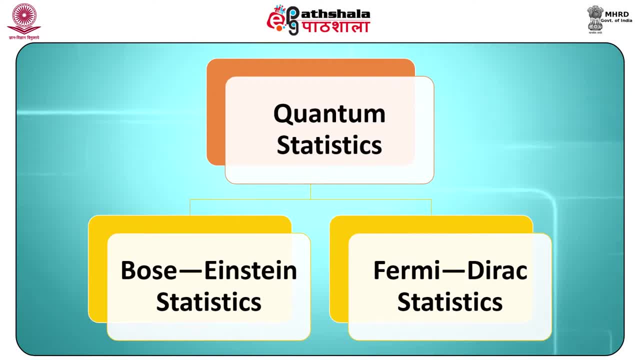 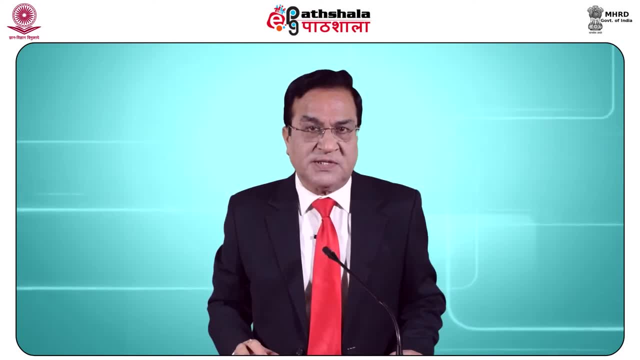 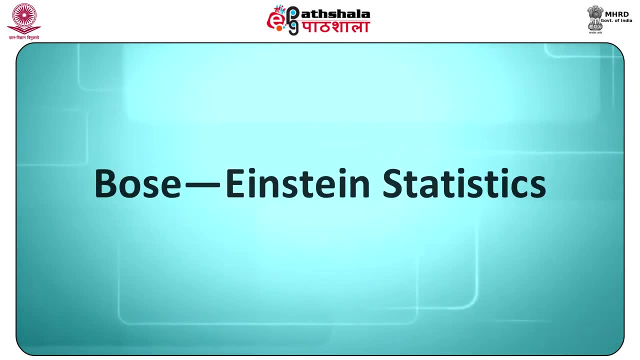 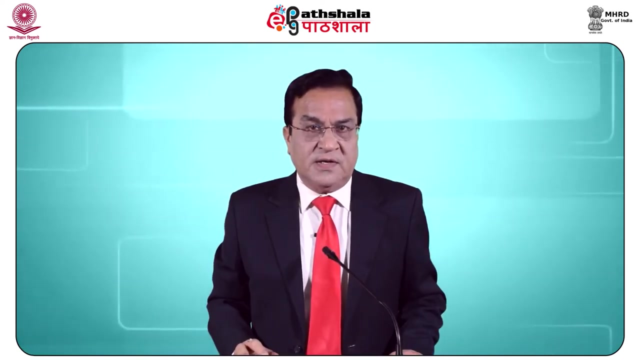 statistics. One is the Bose-Einstein statistics and second is the Fermi-Dirac statistics. For both these statistics we will derive the corresponding distribution laws. In the Bose-Einstein statistics we deal with the particles and take into consideration their internal structure. Now let us look at the Fermi-Dirac statistics. This is a big difference from the earlier Maxwell-Boltzmann statistics. Secondly, particles in the Bose-Einstein statistics are considered indistinguishable from each other and also there is no restriction on the occupancy of the energy levels. 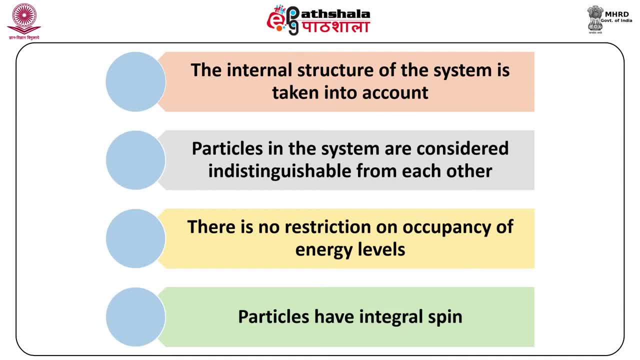 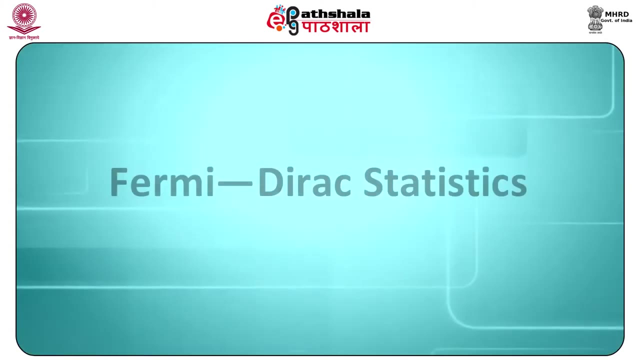 Here one may ask that which type of particles will obey Bose-Einstein statistics? It has been found that the particles which have integral spin, such as photons, they obey Bose-Einstein statistics, and these spin can be calculated once we know their internal structure. On the other hand, in Fermi-Dirac statistics, which we will also study today, 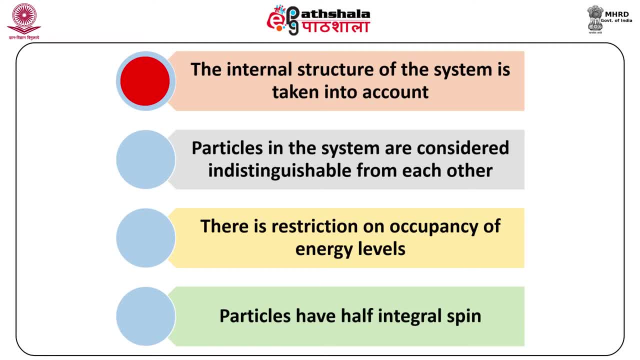 We also take into account the internal structure of the particles. But here the particles, unlike the Bose-Einstein statistics. they have half integral spin like electrons. So if there is a collection of electrons they will obey Fermi-Dirac statistics. These particles are also indistinguishable from each other, and there is here restriction. 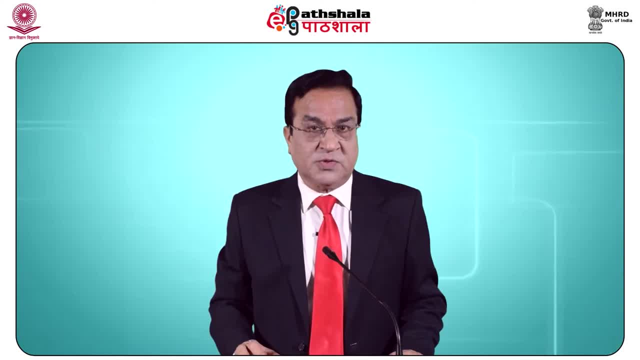 on the occupancy of energy levels. Please note this is very important. in Bose-Einstein statistics there is no restriction, But in Fermi-Dirac statistics, which is obeyed by half integral spin particles, there is a restriction on the occupancy of energy levels. 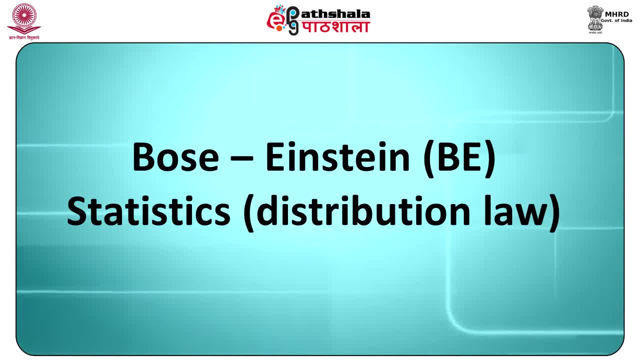 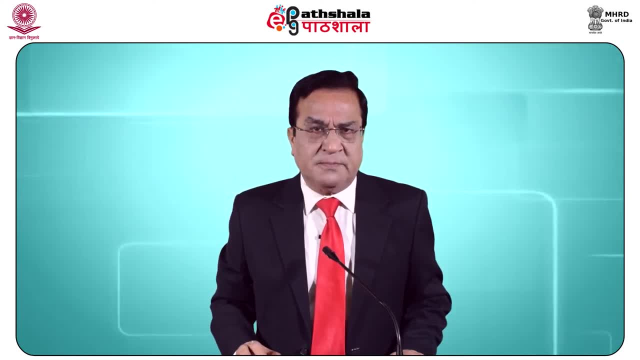 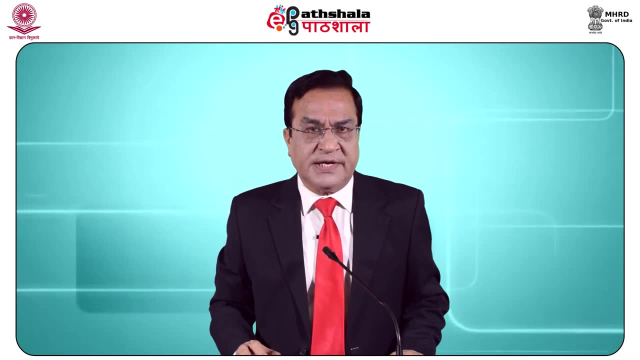 Let us now first derive the Bose-Einstein distribution law. The Bose-Einstein distribution law- basically we mean by deriving the Bose-Einstein distribution law- means we have to find out what distribution will give W the maximum value. That means what value of N i will make the maximum number of microstates possible for. 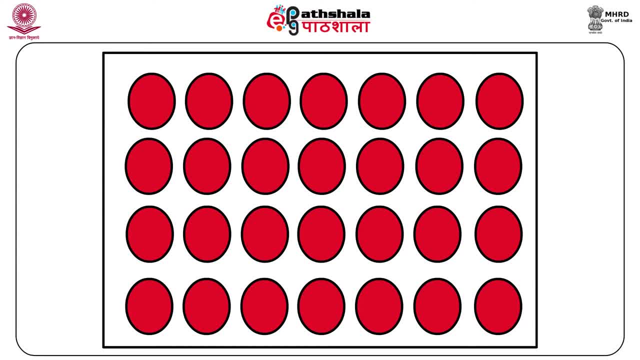 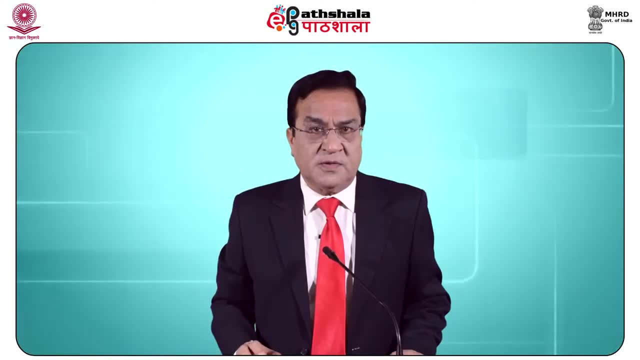 such a system. Here we start with a system which contains N particles. What is N? which obey Bose-Einstein statistics, and the total energy of the system is E, and let the whole system be at temperature T. Now, as we have already learnt earlier, also, if n i 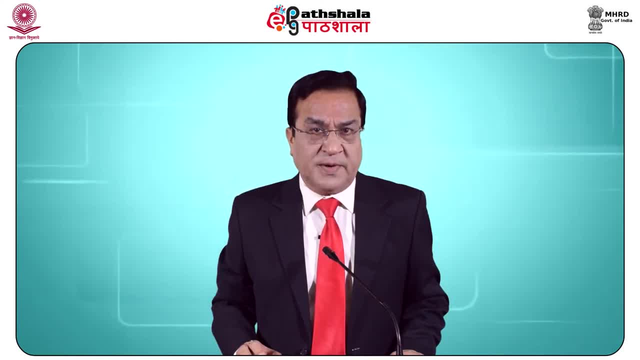 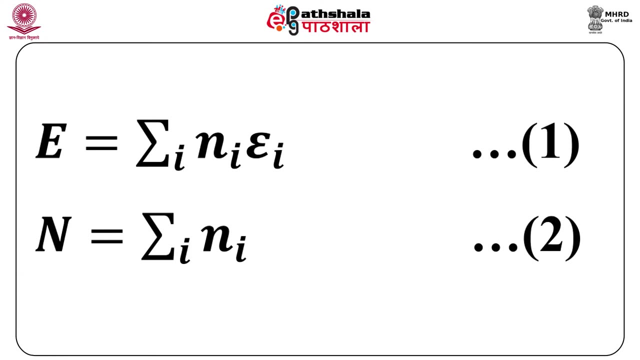 is the number of particles occupying ith energy level with energy epsilon i, and then we can see that the following two conditions must be satisfied: First is equation 1, which gives the expression for total energy, and that is equal to summation n- i epsilon i, and second is capital N, which is equal to summation i n i. Now, as you have, 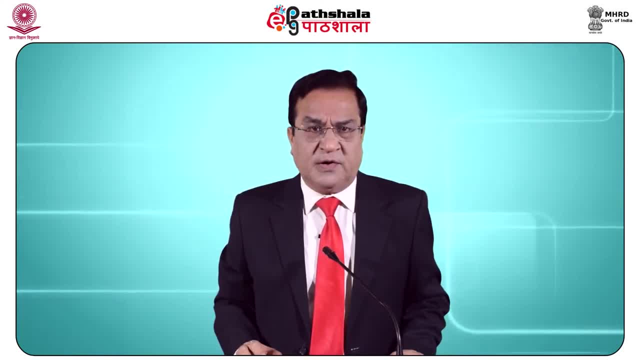 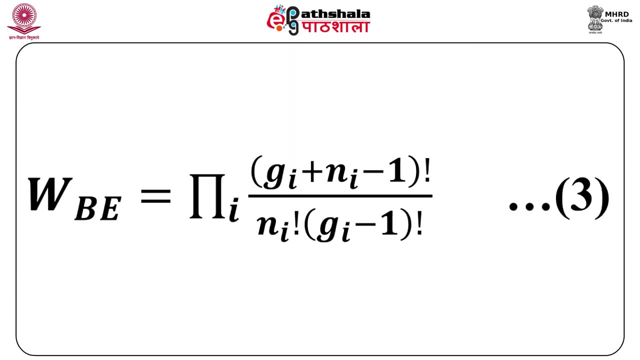 already learnt earlier that the value of W, that means the number of particles occupying microstates associated with any macrostate- in the case of Bose-Einstein statistics, is given by the expression. This is: W. be is equal to pi i, that is the capital, pi i, which is 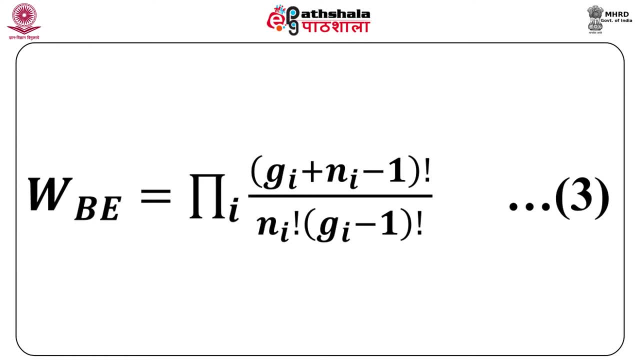 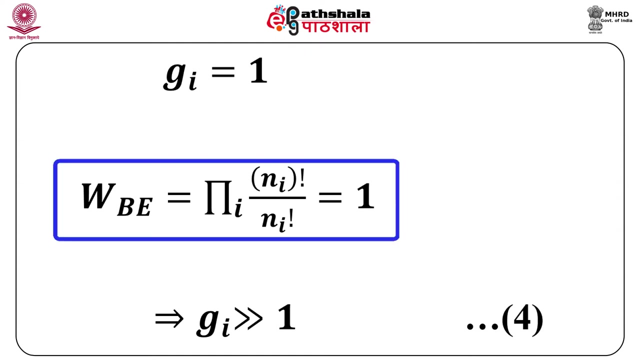 equal to g i plus n i minus 1 factorial, divided by n? i factorial, then g i minus 1 factorial, Then in that case W, b, a, e, as you can see here, will reduce to 1. that means there will be no microstate, that means only one microstate associated with any macrostate. So in this 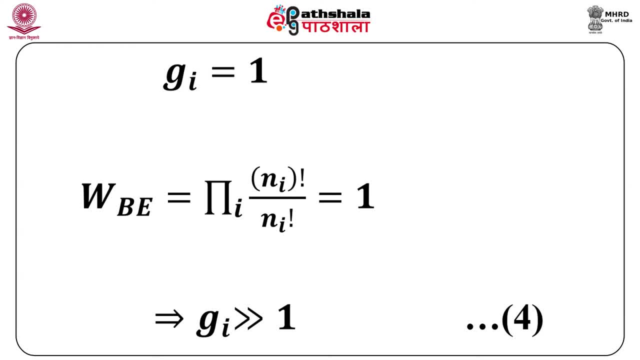 case, the number of microstates arise primarily because of the degeneracy of the energy levels. So degeneracy plays a very, very important role in Bose-Einstein statistics. 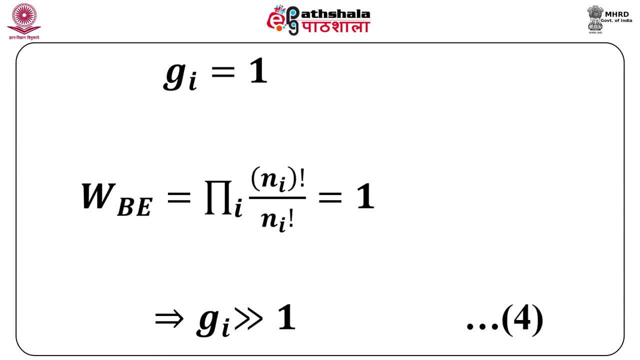 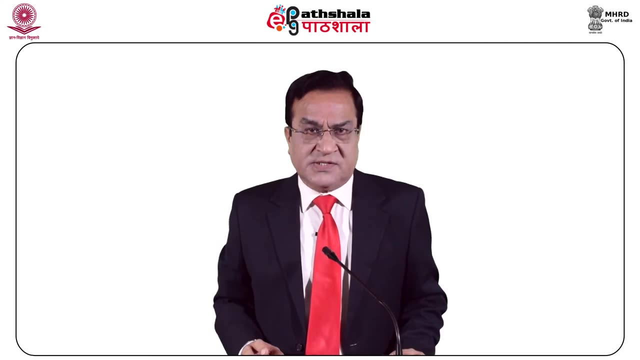 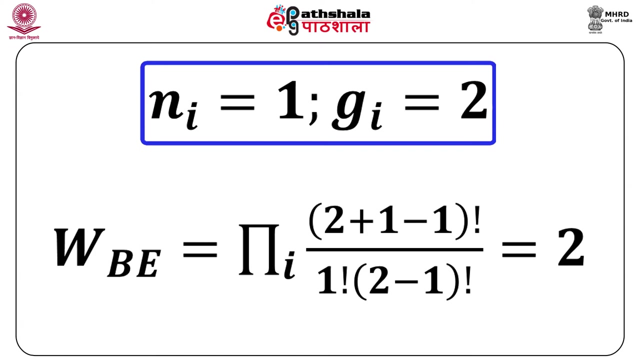 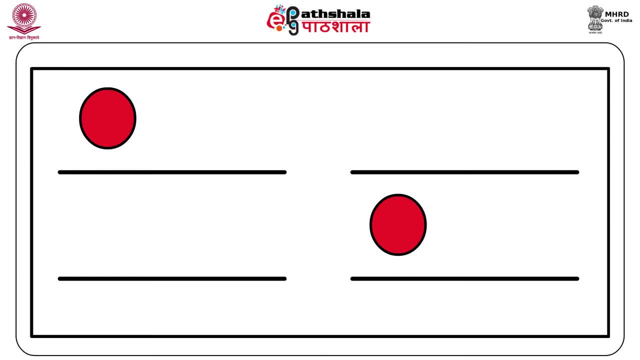 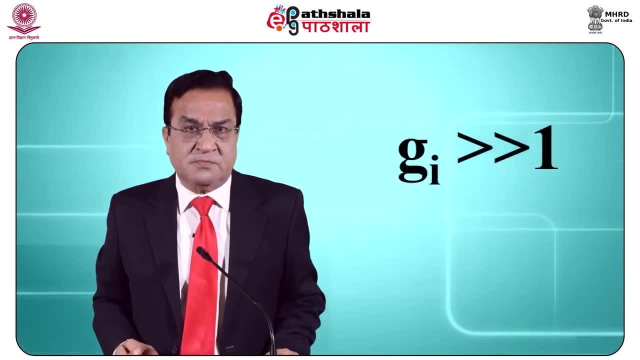 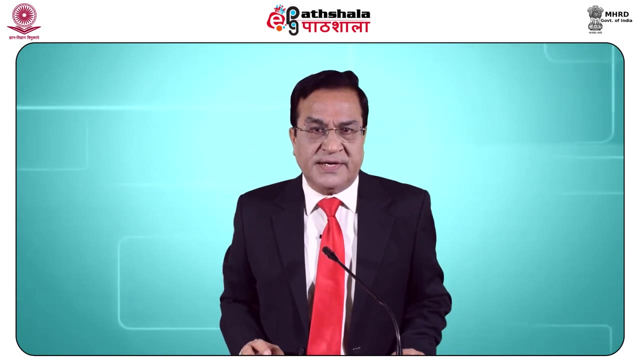 Since there are two ways in which the distribution of the given particle can be achieved in the two specified states given by the Gi value. Now, since in the Bose-Einstein statistics generally Gi is much, much greater than 1, therefore the expression for W can be simplified and it can be written as it is shown in equation. 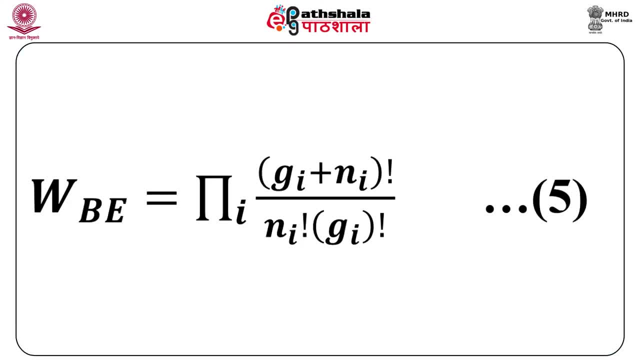 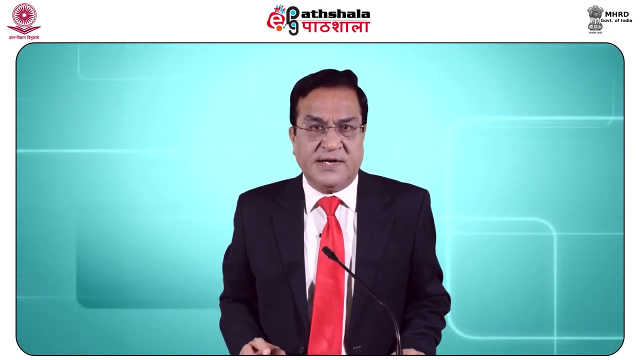 5. Wb is equal to pi. i is equal to Gi plus Ni factorial divided by Ni factorial, Gi factorial. We have neglected 1 in comparison to the rest of the terms, because Gi is much, much larger than 1.. Now if we have to find out the value of Ni which will make Wb maximum, we will proceed. 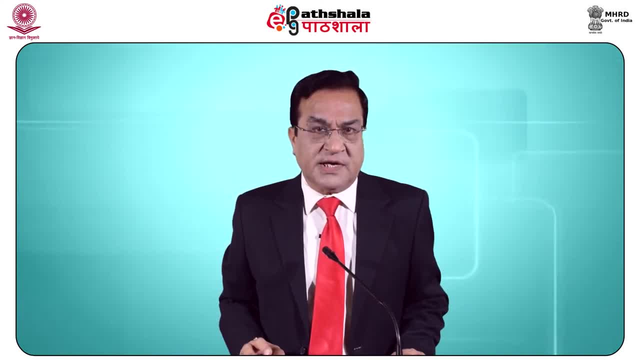 exactly in the similar way as we have done in the case of Maxwell-Boltzmann statistics. First thing which we do is we take logarithm on both sides. but before doing that, we have already done it in our Maxwell-Boltzmann statistics, and that is that dE will come out to be equal. 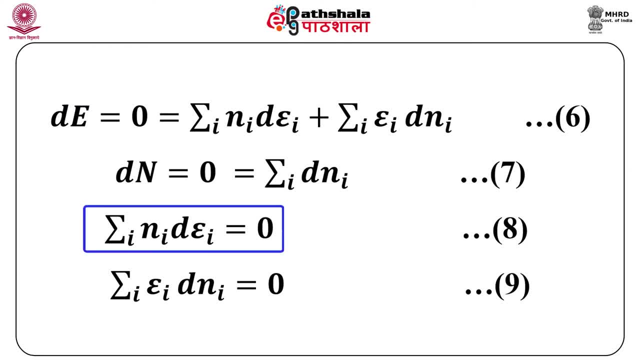 to 0 and that will make summation Ni, d epsilon i is equal to 0.. That is basically equation 8, as we have seen here. and then there is equation 7, which come once we take the differential of N capital, N dN becomes 0, and that is summation i dNi. 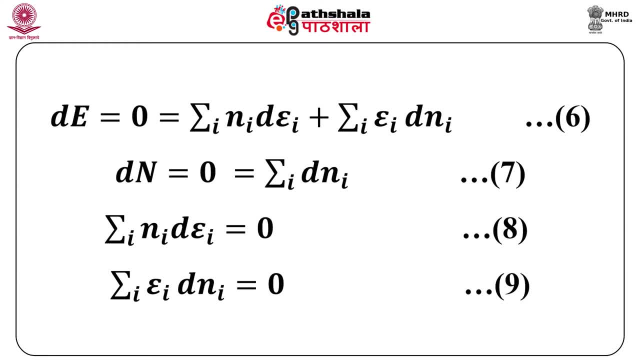 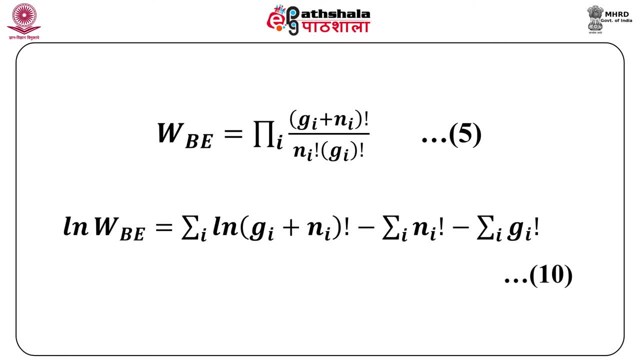 is equal to 0.. So these two equations were there in our Maxwell-Boltzmann statistics as well. Now we take the logarithm of the expression for WbE and this gives us equation 10, which is ln. Wbe is equal to summation i ln Gi plus Ni factorial, minus summation i, Ni factorial. 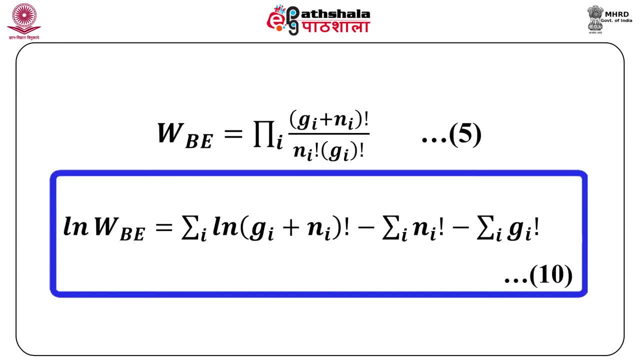 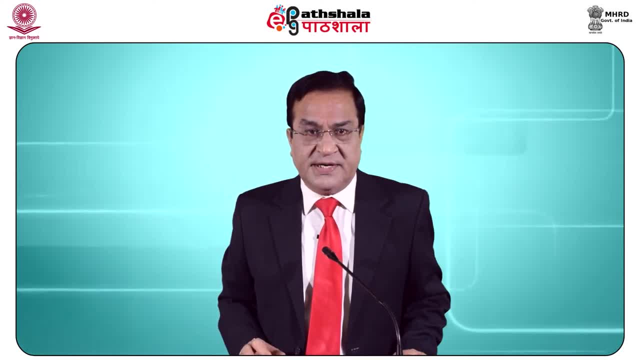 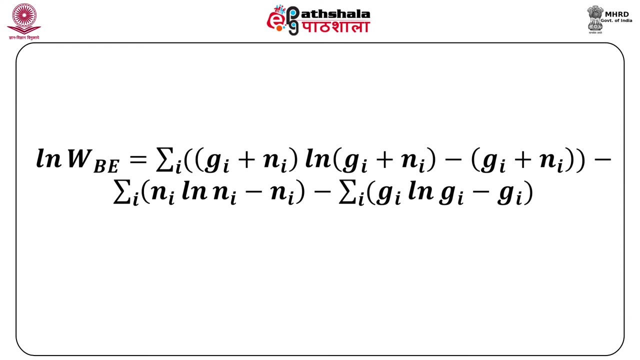 minus summation i Gi factorial. Here also we now apply the Stirling approximation, which we have learnt already. and once we use the Stirling approximation, this equation gets modified and we get the following relation, as it is shown here: ln Wbe is equal to summation i Gi plus Ni ln Gi plus Ni minus Gi plus Ni parenthesis. 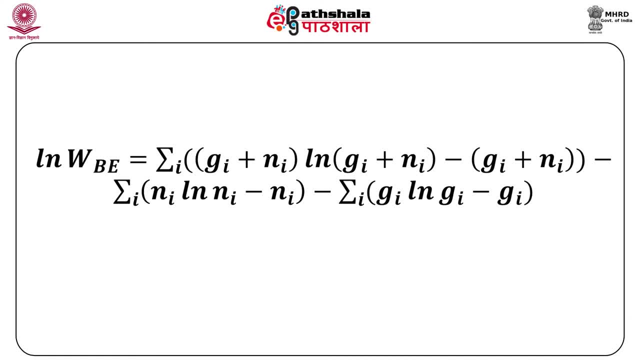 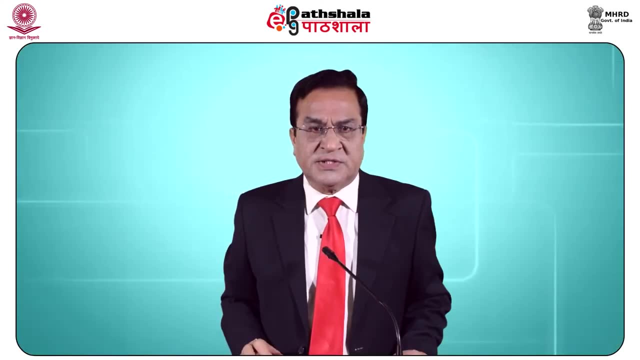 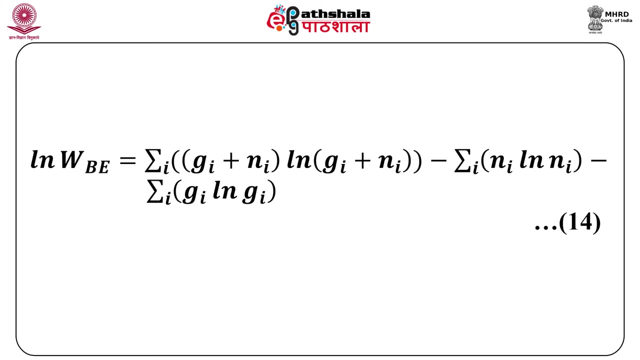 closed. minus summation: i Ni ln Ni minus Ni minus summation i Gi ln Gi minus Gi. This equation has come after applying the Stirling approximation. This equation And simplification gives us the equation as you can see here. This gives ln. Wbe is equal to summation i Gi plus Ni ln Gi plus Ni. minus summation i. 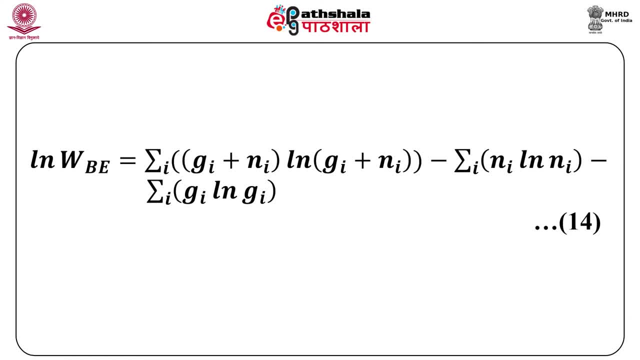 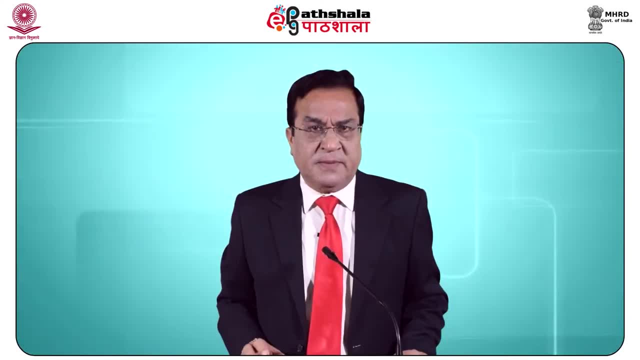 Ni ln Ni. minus summation, i Gi ln Gi, and that is equation 14.. So this we have obtained by applying Stirling approximation And of course, initially we took logarithm. Now we apply the first condition of maxima, and that is d ln. W should be equal to 0. 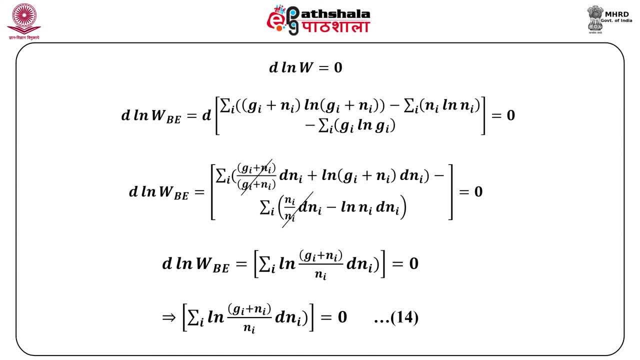 And if we apply this condition as we have done it here, we get ultimately: d ln Wbe is equal to summation i ln Gi plus Ni upon Ni and d Ni is equal to 0, or in other words, summation i ln Gi plus Ni upon Ni is equal to 0.. 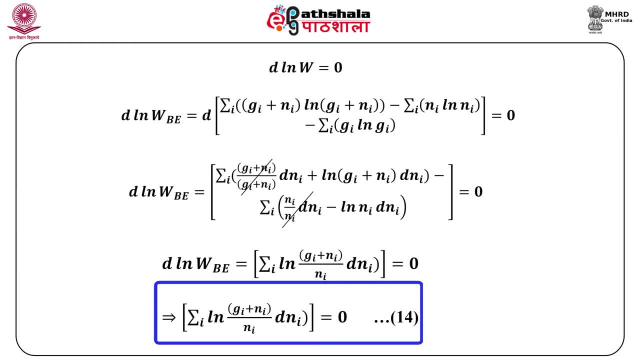 Now say we transcriptilize this And then we get that can be expected, as d in j is equal to 0 and d in j is equal to 15.. So if we use� so, we get then d in less than or equal to, in less than or equal to 0 and 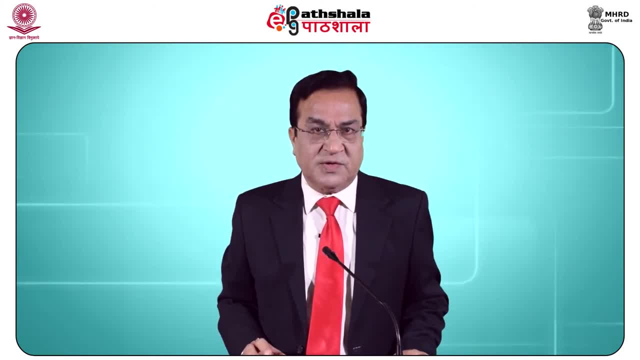 then d is equal to, in less than and not equal to or equal to any of the statisti question f. Now, if we look at above the equation, If we uhh practise, So at first I just want to feel three equations for each hypothesis. The first one is: wbe is equal to 0 and d is equal to 0 and d mi d. 1 into d? n is equal to 0, and new is innovation y operation★. and then d death I into d? n equal to zero. 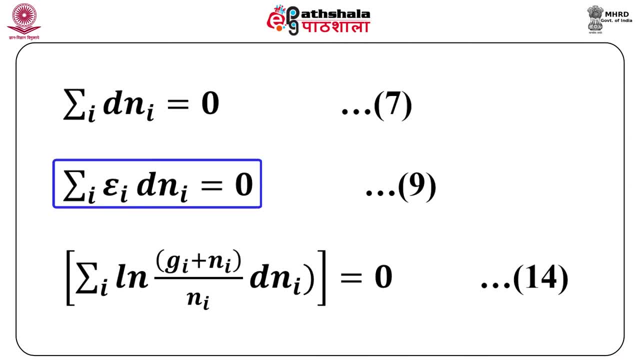 This is the third equation, equation number 14, which we get. So in all we have 3 equations now, As we had in the case of maxm Dragel Boltzmann statistics. Second is summation. epsilon i, d, n, i is equal to 0. that is equation 9, and then summation. 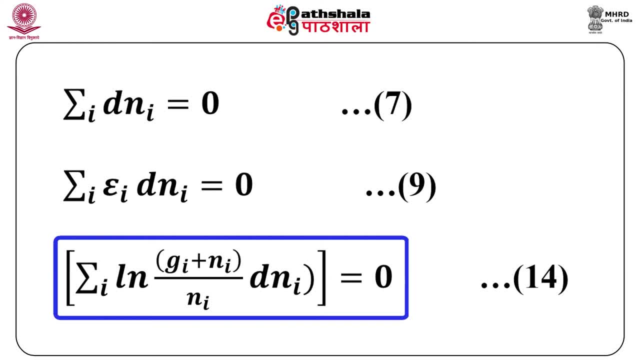 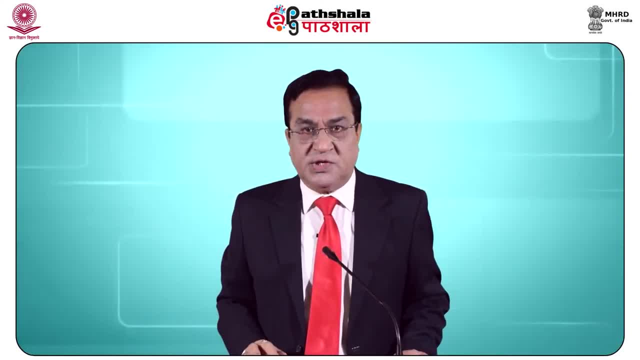 i, ln, g, i plus n, i, divided by n, i into d, n, i, is equal to 0. that is equation 14.. Now again, these three are independent equations, each one of them equal to 0. they can be combined for a given system using Lagrange's method of undetermined multipliers. 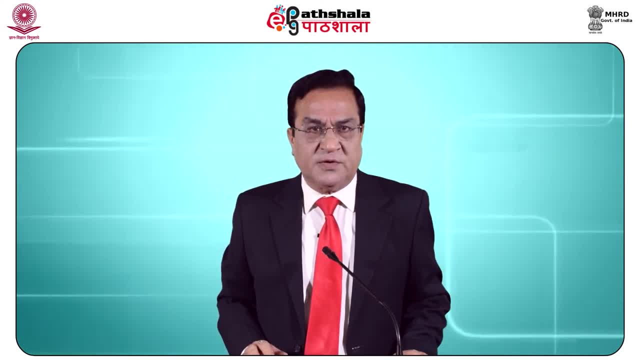 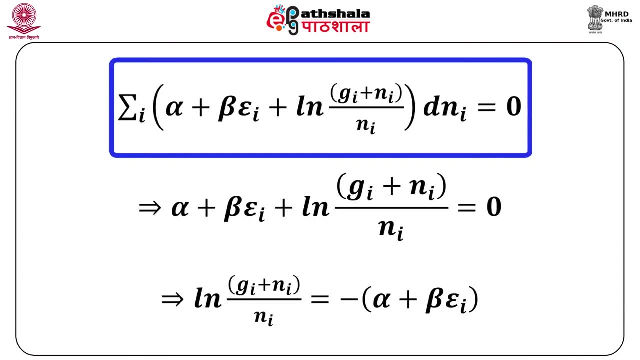 We multiply one equation by alpha, other with beta, as we did it earlier in the last module, and we get the corresponding equation summation. i is equal to alpha plus beta. epsilon, i, ln, g, i plus n, i upon n i- parenthesis close- d n, i is equal to 0.. 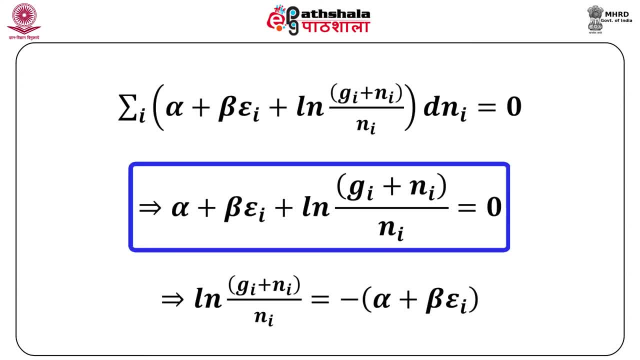 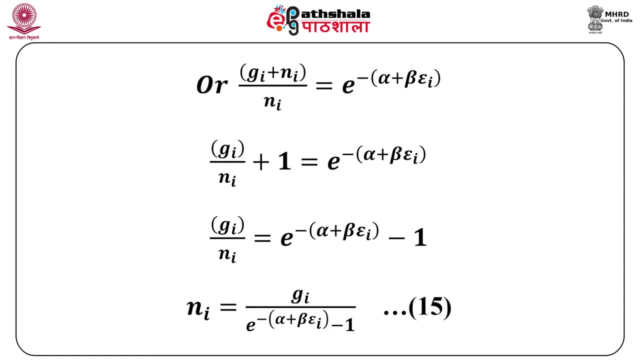 And in this equation we can notice that alpha plus beta epsilon i plus ln, g, i plus n i upon n i would be equal to 0. So for each value of i and if we simplify it, one gets the following expression, which is: n. i is equal to g i divided by e to the power, minus alpha plus beta epsilon i minus. 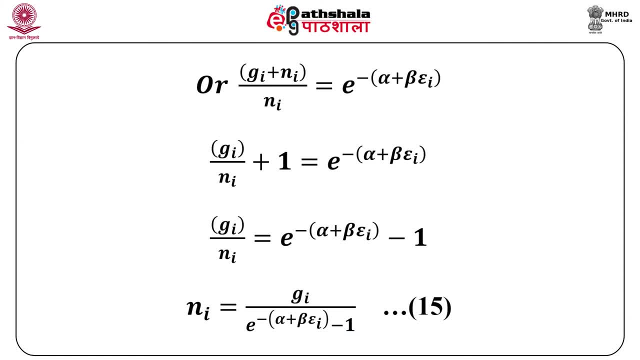 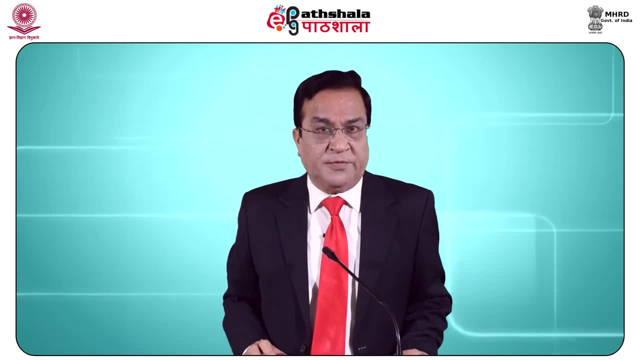 1, that is equation 15.. So this equation gives us the Bose-Einstein distribution law, although alpha and beta are still unknown, But as we will see later on. here also, beta will come out to be equal minus 1 upon k, t, and similarly alpha- we will show this also- is the corresponding partition function. 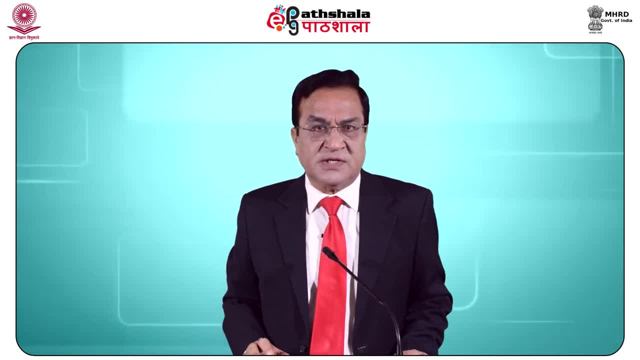 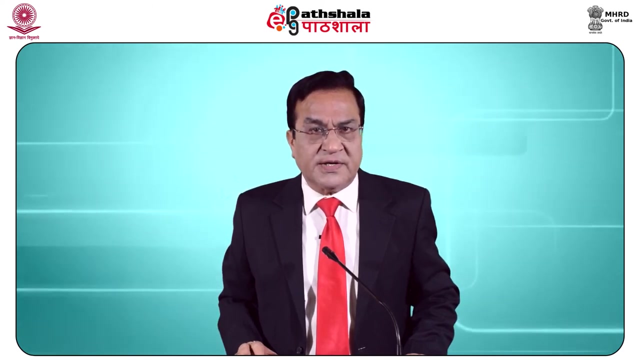 And this Bose-Einstein distribution law gives us the value of n i which, when substituted in the expression for w be, will make w be maximum. That means it gives the value for the most probable macrostate for Bose-Einstein statistics. After having derived Bose-Einstein distribution law exactly on similar lines, one can go ahead. 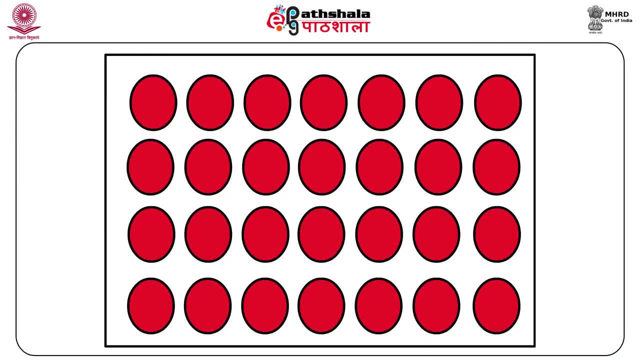 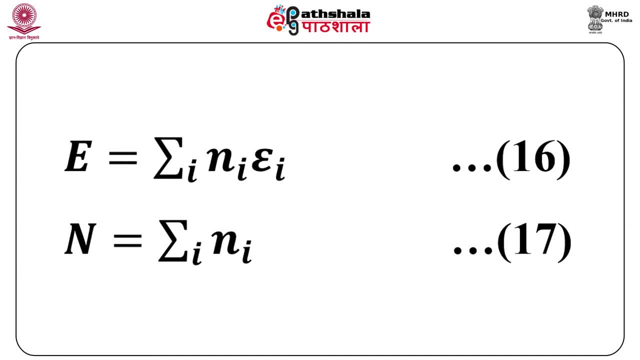 for Fermi Dirac distribution law. Here also the total e and total n. they are constant And they are given by the expression: E is equal to summation i n, i, epsilon i and capital N is equal to summation i n, i. 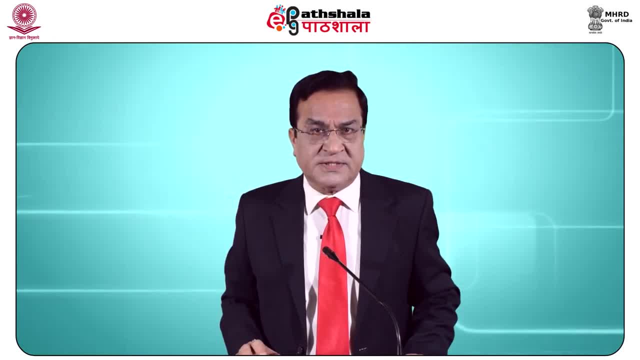 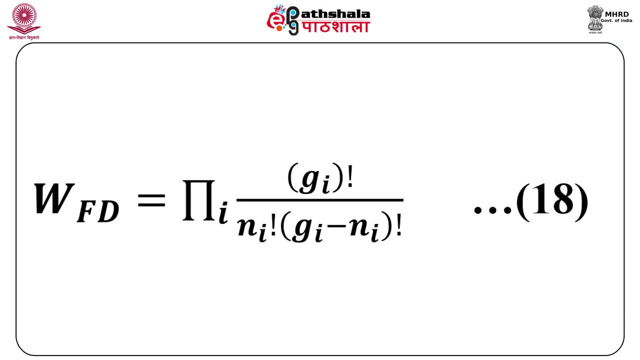 The value of the w for Fermi Dirac statistics, as we have already learnt in our second module, that is given by WFD, is equal to pi i g i factorial divided by n? i factorial. g i minus n? i factorial. This is the equation 18.. 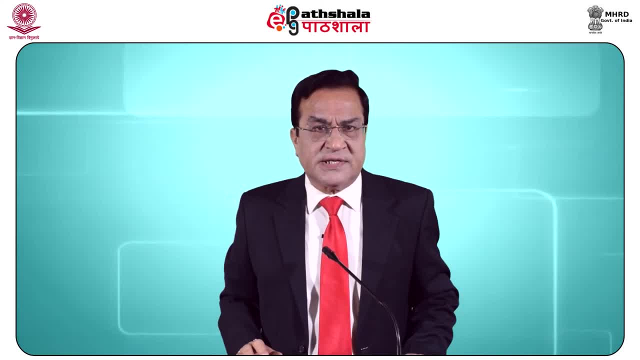 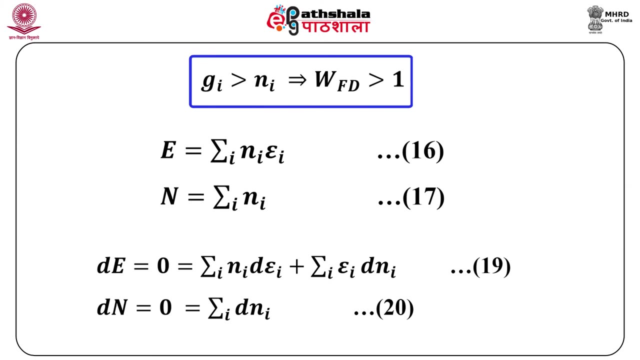 Here also, as you will notice here, that the degeneracy will play a very, very important role, and one can see that for getting a meaningful value of WFD, g i should be greater than n? i, because if g i is greater than n? i, then WFD would be greater than 1.. 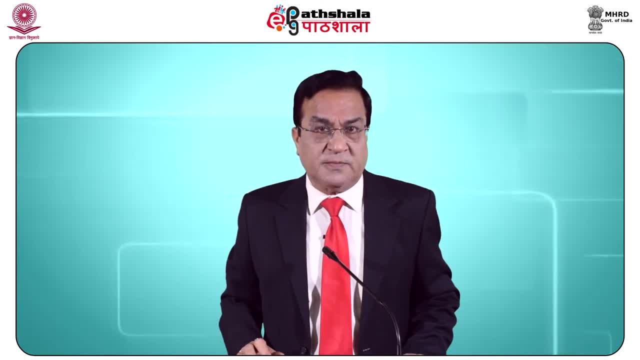 However, if g i is equal to n i, as you can see from expression 18.. This whole expression will reduce to 1. that means just one microstate for every macrostate. So here also the degeneracy is going to play a very, very important role. 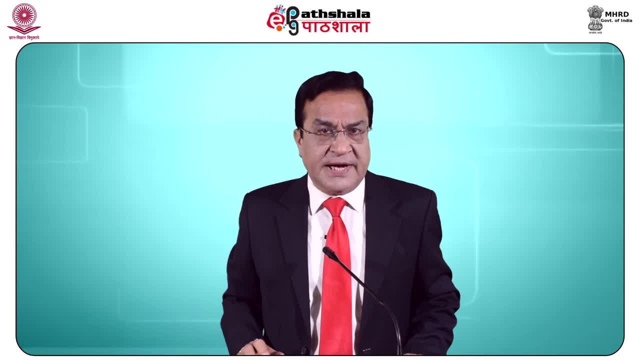 Here also we need to find out that value of n? i which, when substituted in the expression for WFD, will make WFD maximum. We take the differentials of the two equations. First equation, As we derived it earlier, is equation 20, which is summation i, d, n i is equal to 0, and second: 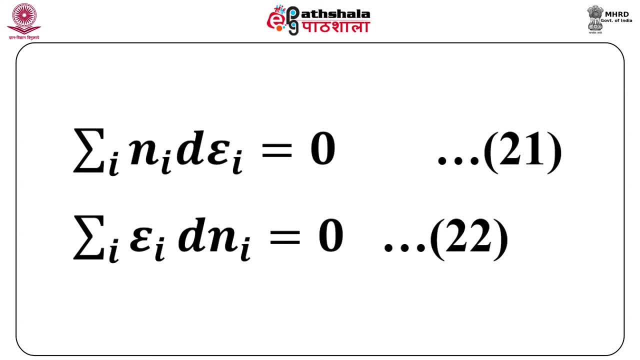 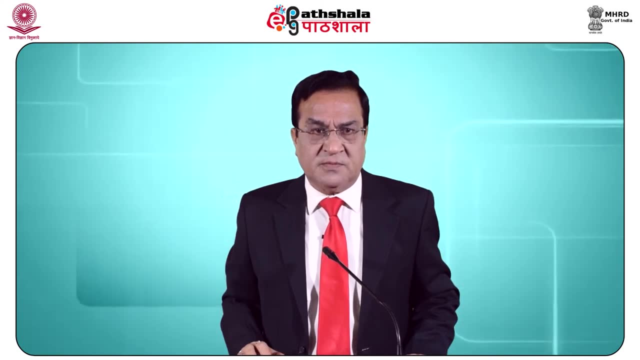 which comes from the constant value of energy, and that is summation i, n, i, d epsilon i is equal to 0. This, ultimately, will give us the equation: summation i, epsilon i, d n i is equal to 0.. Exactly on the similar lines. now we take the logarithm of WFD. 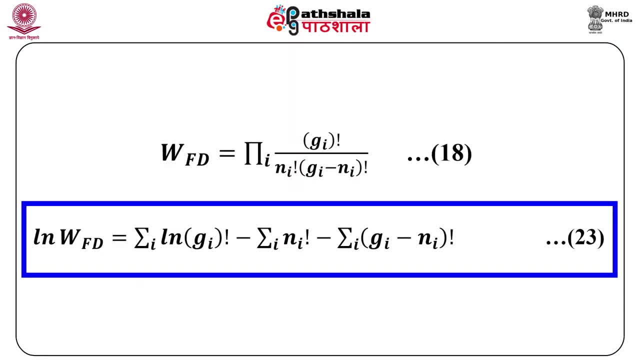 So if we do that We get ln FD is equal to 0.. If we take the logarithm, of WFD is equal to ln summation i, ln, g, i factorial minus summation i, n i factorial minus summation i, g i minus n? i factorial. that is equation. third. 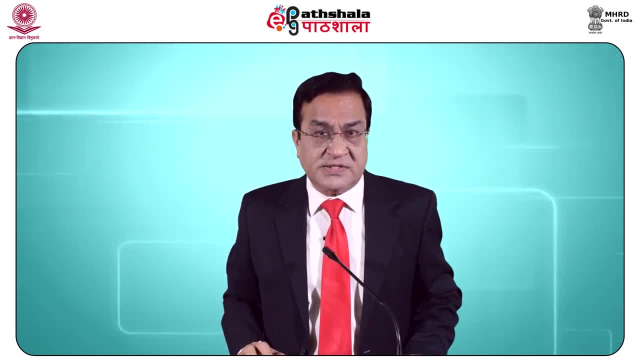 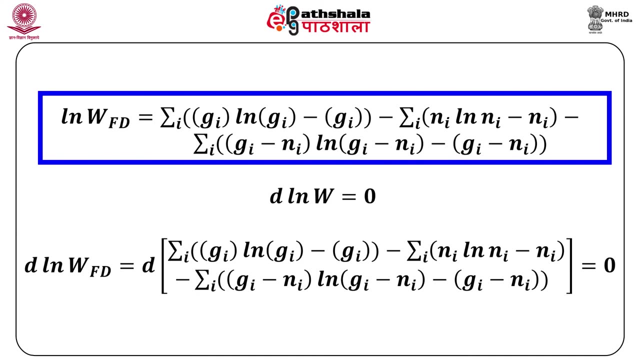 We simplify it further by applying once again sterling approximation and using simplifying it, We get the expression which you can see is that ln. WFD is equal to summation i, d, n, i is equal to 0.. If we do that, We get the expression which you can see is that ln. WFD is equal to summation i, g, i, ln. 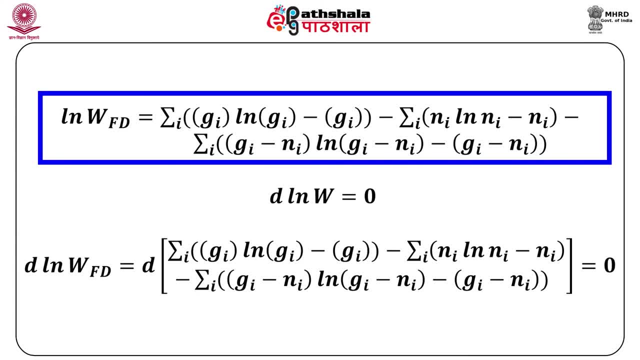 g i minus g i, parentheses closed. minus summation: i n i, ln, n i minus n i, parentheses closed. minus summation: i g i minus n i, ln, g i minus n. i minus g i minus n i, parentheses closed. And if we apply the first condition of maxima here once again, then the first differential 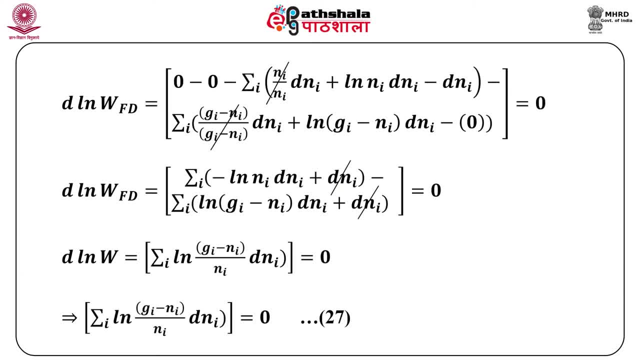 should be 0. And once we do that, As we are doing it here, you can see d ln WFD and if we simplify it further, ultimately we get the equation 27, which comes from the fact that d ln W comes to be equal to summation. 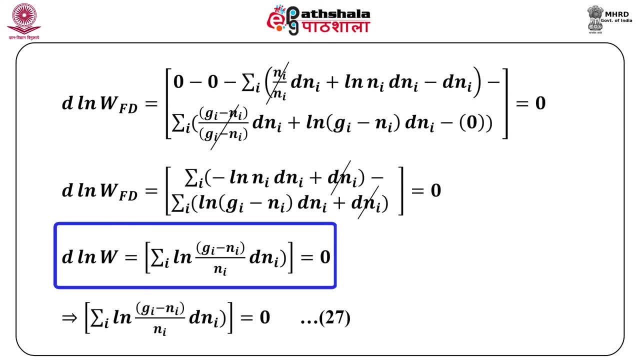 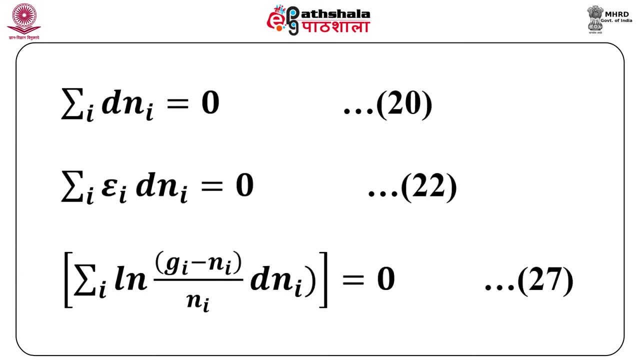 i ln g i minus n? i upon n? i d n i is equal to 0, or in other words, summation i ln g i minus n? i upon n? i d n i is equal to 0.. So once again we have these three equations. 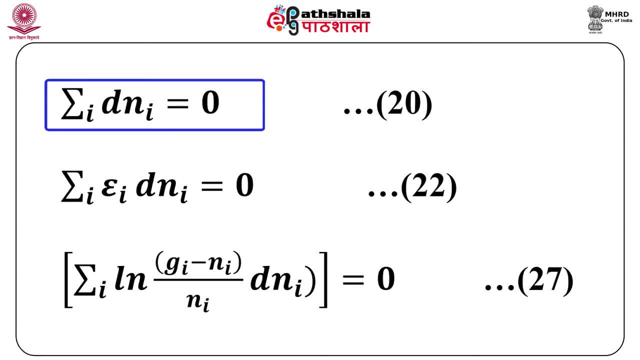 First equation comes from the constant value of n. Second equation comes, which is 22nd. that comes from the constant value of e, and the third, which is 27. that equation comes from applying the first condition of maxima, That means the first differential. 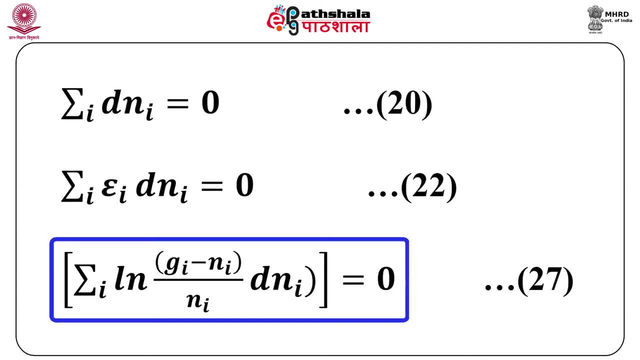 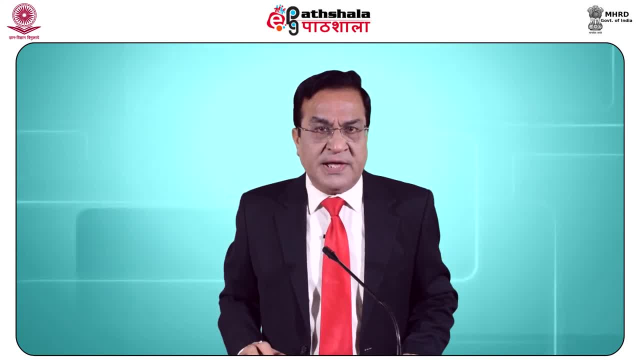 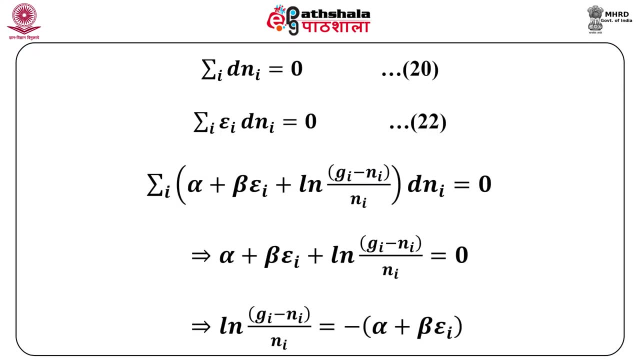 That means the first differential. That means the first differential is taken to be equal to 0. And if we have these three independent equations, applying the method of Lagrange's method of undetermined multipliers, and we combine these three equations, we get ultimately as we have. 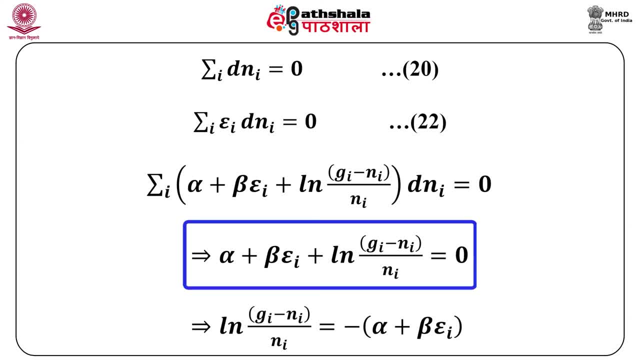 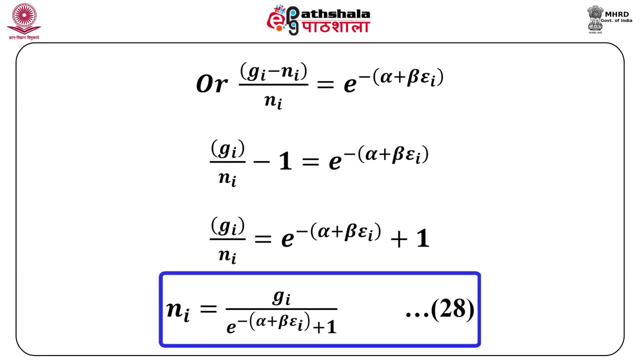 done it earlier, it comes to be alpha plus beta, epsilon i plus ln, g. i minus n. i upon n i is equal to 0. For each value of alpha, For each value of alpha, For each value of i, And this, on simplification, gives us n. i is equal to g i upon e, to the power minus alpha. 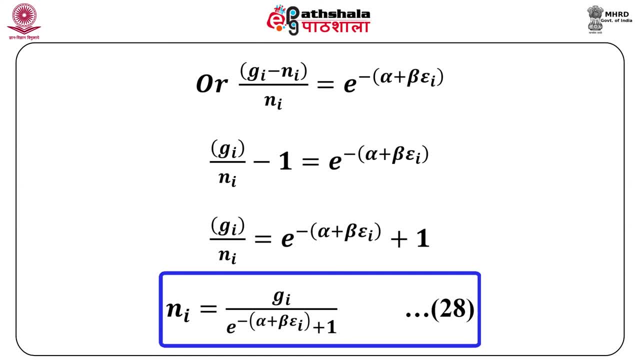 plus beta, epsilon i plus 1, and that is the equation 28.. And this gives us what is known as the Fermi Dirac distribution law. That means this value of n? i which we get from equation 28.. If this is such, 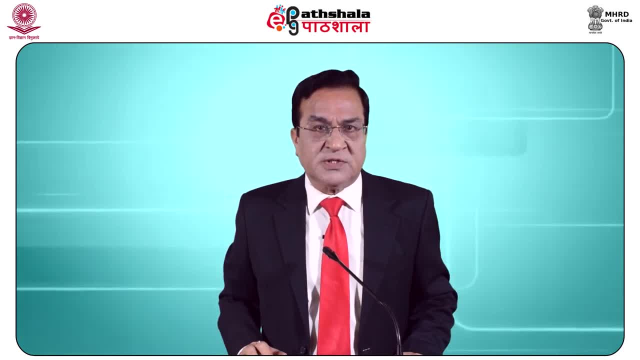 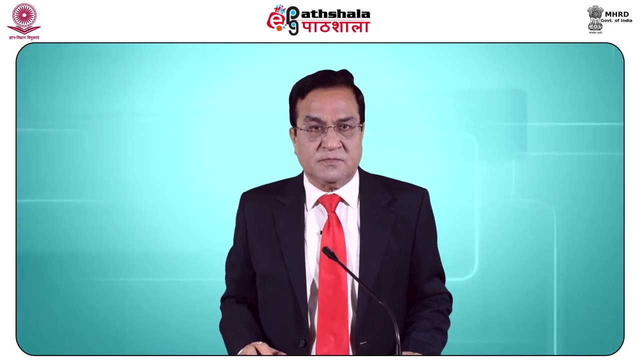 If this is such, If this is substituted in the expression for WFD, then it will make WFD maximum and hence it will be the most probable macrostate for Fermi Dirac statistics. As here also we can show, beta will come out to be minus 1 upon kT and alpha is nothing. 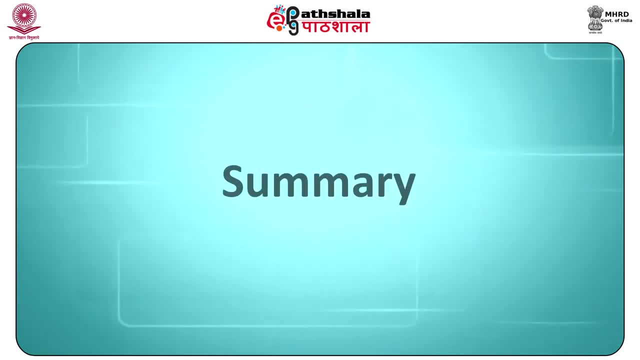 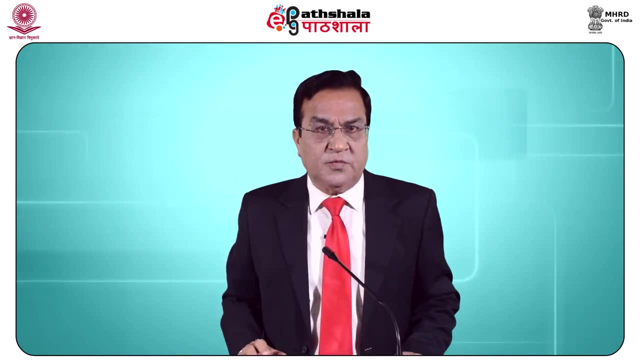 else but the partition function. So in this module we have gone into the details of quantum statistics. Quantum statistics basically deals with those particles where we take into account the internal structure. There are two types of quantum statistics. one is the Bose Einstein statistics, which is applicable to integral spin particles. 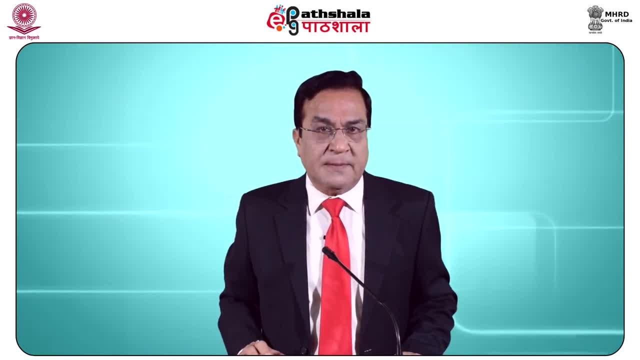 And second is the Fermi Dirac statistics, which is applicable to half integral particles. In the case of Bose-Einstein statistics, there is no restriction on the occupancy, whereas in the case of Fermi Dirac statistics, there is a restriction on the occupancy And in for both of these statistics we have derived 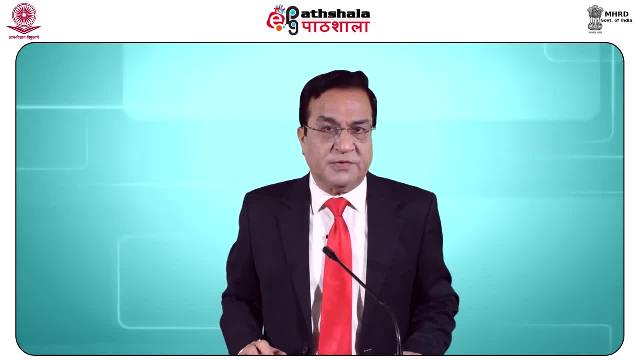 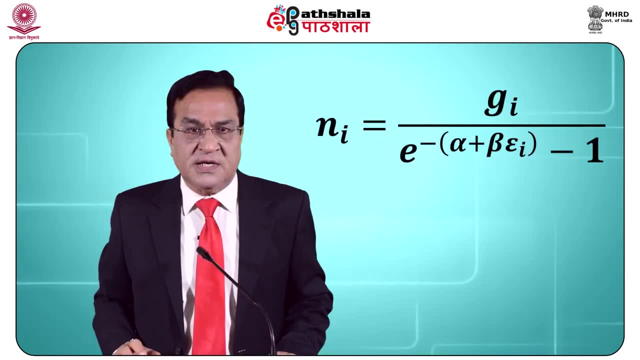 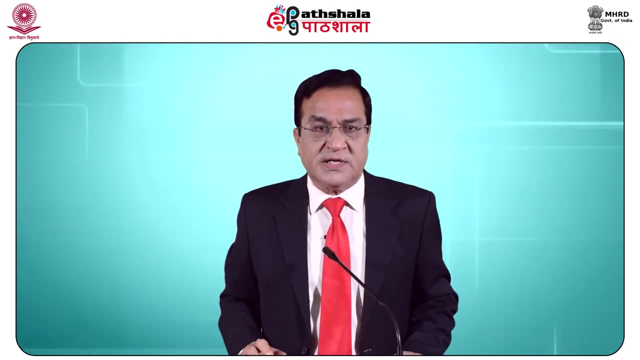 the corresponding distribution laws, which will give us the maximum value of W For Bose-Einstein statistics. this law gives: n. i is equal to g, i e to the power minus alpha plus beta, epsilon i minus 1.. Whereas for Fermi Dirac statistics, n i comes. 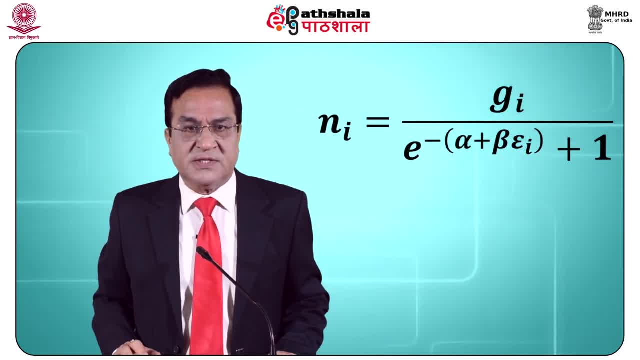 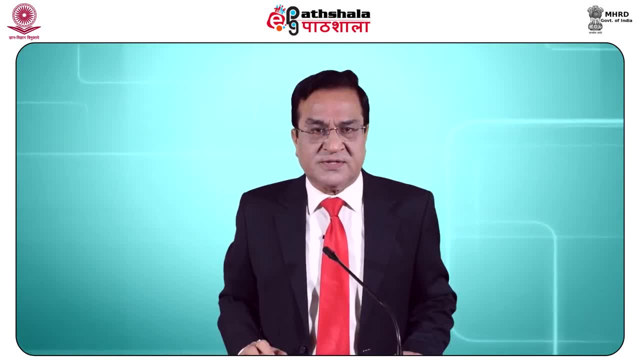 to be equal to g, i upon e, to the power minus alpha plus beta, epsilon i plus 1.. If you examine them closely, in Bose-Einstein statistics in the denominator there is a minus sign minus 1. Whereas in the Fermi Dirac statistics it is the plus sign. So that is very easy to remember.